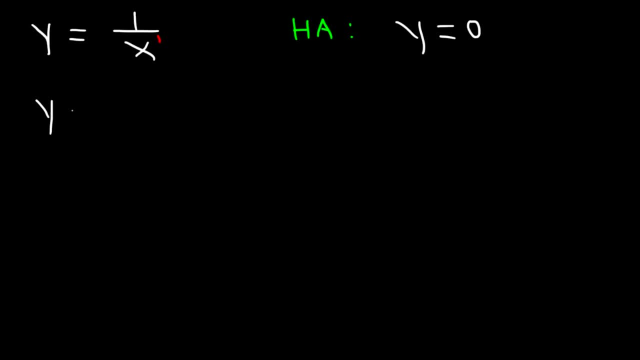 So let's try this example: 7 over x minus 3.. The degree of the denominator is 1,. the degree of the numerator is 0, so it's bottom heavy. therefore, the horizontal asymptote is: y is equal to 0.. 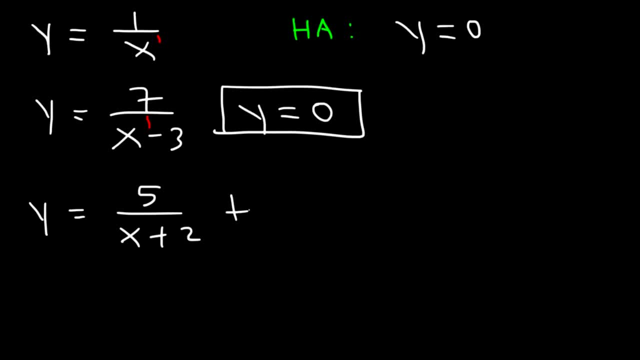 Now what about this one, 5 over x plus 2 plus 3?? So if you just look at 5 over x plus 2, it's bottom heavy. so it's y equals 0 for that plus 3.. But notice that 3 is added to it. 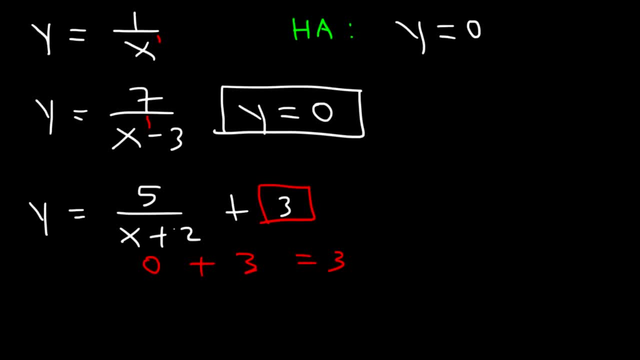 So 0 plus 3 is equal to 3.. So the horizontal asymptote is: y is equal to 3.. Now what about this one: 8x minus 6 over x squared plus 3x. So notice that this function is bottom heavy. 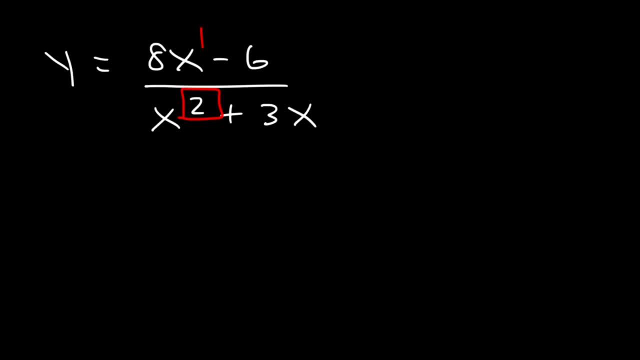 The degree of the denominator is 2, the degree of the numerator is 1, so it's going to be y is equal to 0. Because it's bottom heavy, Now let's say if we add a negative 9 to it, it's going to be 0 minus 9.. 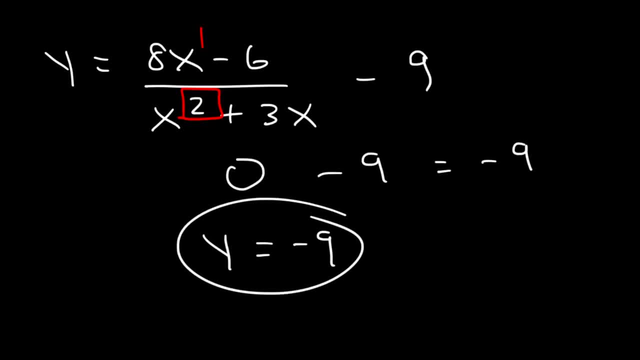 So the horizontal asymptote is now: y equals negative 9.. Now what about this one? Let's say 2x minus 3 divided by x plus 4.. What do you think the horizontal asymptote is going to be? So notice that the degree of the numerator is the same. 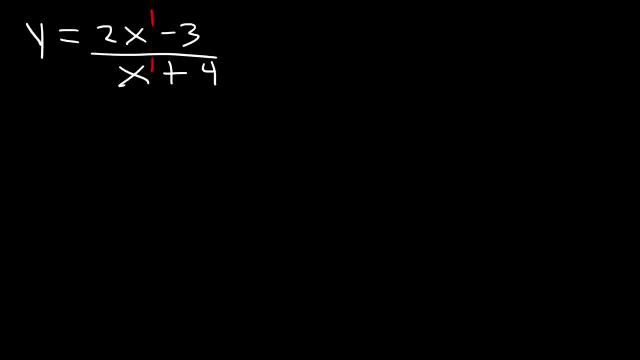 It's the same as that of the denominator, So it's neither top heavy nor bottom heavy. In a situation like this, divide the coefficients. So 2 divided by 1 is 2.. So therefore the horizontal asymptote is: y is equal to 2.. 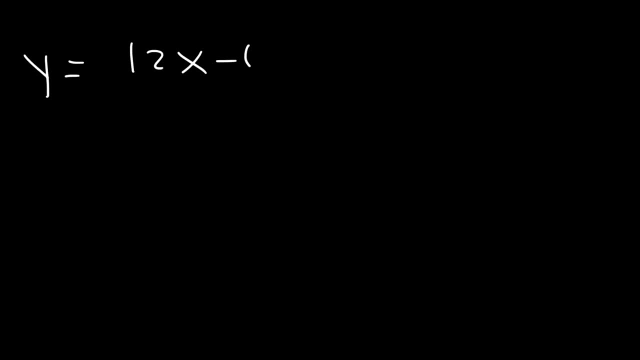 Try this one. Let's say, if you have 12x minus 6 divided by 3x plus 4 plus 2.. What do you think the horizontal asymptote is going to be? It's going to be negative: 9 plus 2.. 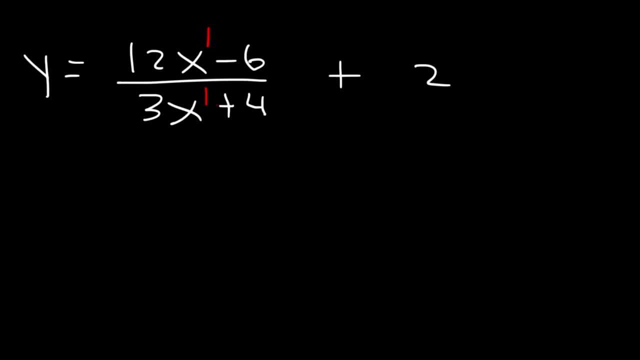 So, as you can see, the degree of the numerator is the same as that of the denominator, So you divide the coefficients that are attached to those variables, So it's going to be 12 over 3, plus the 2 that we see here. 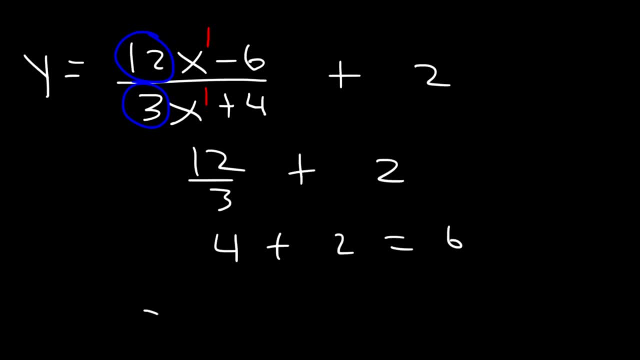 12 over 3 is 4.. 4 plus 2 is 6.. So the horizontal asymptote is: y equals 6.. Try this one: 5 minus 8x squared, That's negative 9.. So the horizontal asymptote is: y is equal to negative 9.. 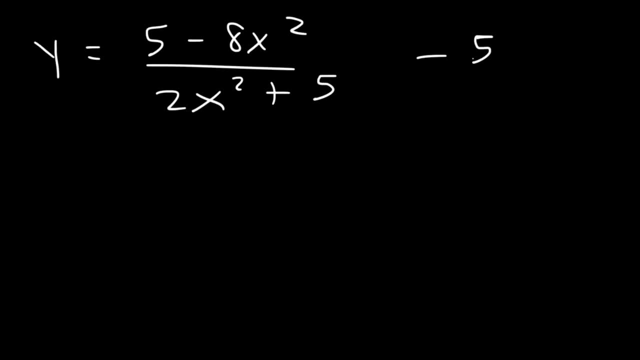 So it's going to be negative. 8 divided by 2x, squared plus 5.. And then minus 5 on the outside, So we can see that the degrees of the top and the bottom are the same. So let's divide the numbers in front of those variables. 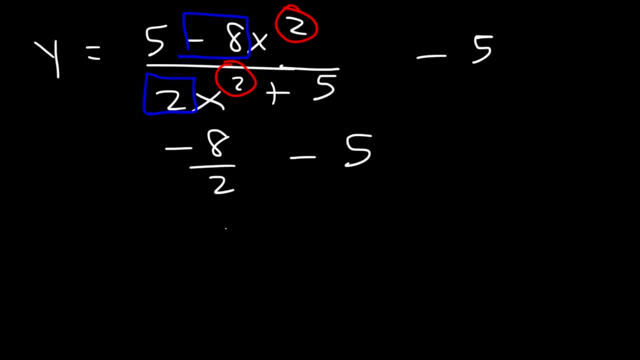 So it's going to be negative 8 divided by 2 minus 5.. That's negative 4 minus 5, which is negative 9.. So the horizontal asymptote is: y is equal to negative 9.. So here's another problem. 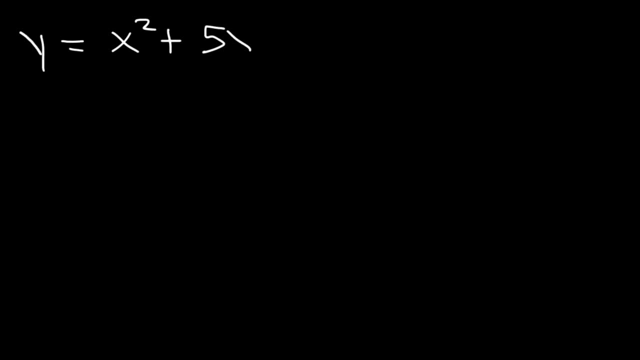 Let's say that y is equal to x squared plus 5x plus 6 divided by x plus 3.. What is the horizontal asymptote? So the degree of the numerator is 2, and the degree of the denominator is 1.. 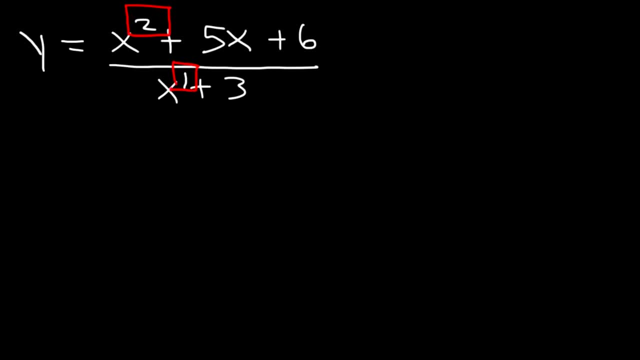 So it's top heavy. Whenever it's top heavy, there is no horizontal asymptote, So it's top heavy. So it's top heavy. But is there a slant asymptote If the degree of the numerator exceeds the denominator by exactly 1,? 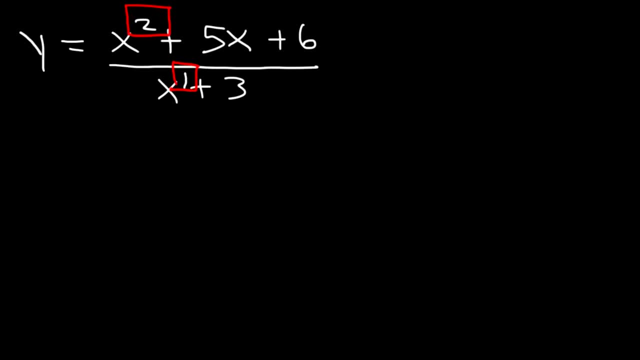 then there is a slant or an oblique asymptote If the numerator exceeds the denominator by more than 1, there is no slant asymptote or oblique asymptote. So how do we go about finding the slant asymptote? 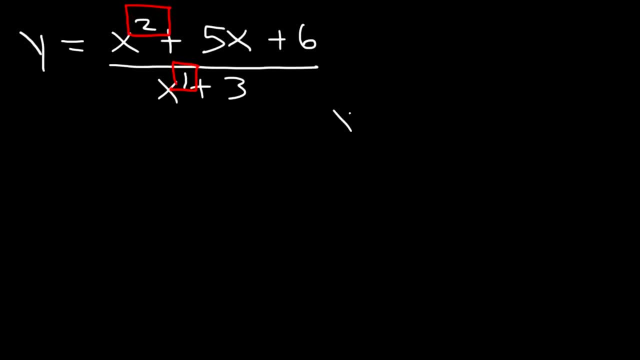 In order to find it you need to use long division, So we have to divide. The numerator is going to go on the inside, So let's divide this number- I mean that variable- by x. So x squared divided by x is x. 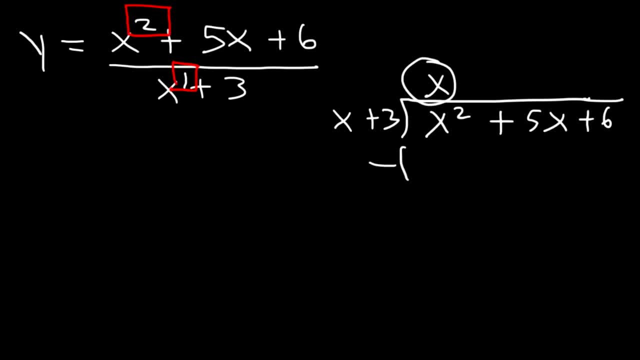 Next: multiply: x times x is x squared. x times 3 is 3x. After that, subtract So x squared minus x squared, That's going to be x squared, That's going to be 0.. And then we have 5x minus 3x. 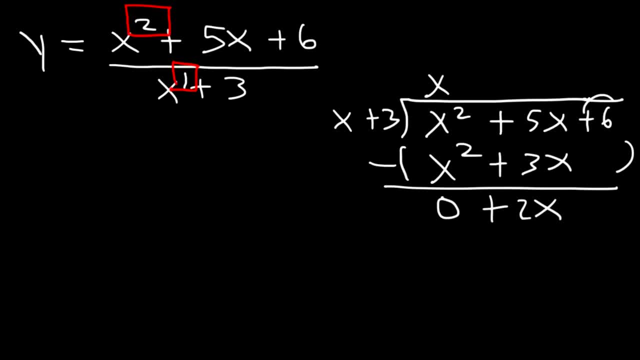 So that's going to be positive. 2x And 6 minus nothing, or 6 minus 0, is simply 6.. So we could just bring down to 6.. And now let's divide again: 2x divided by x, well, that's going to be just 2.. 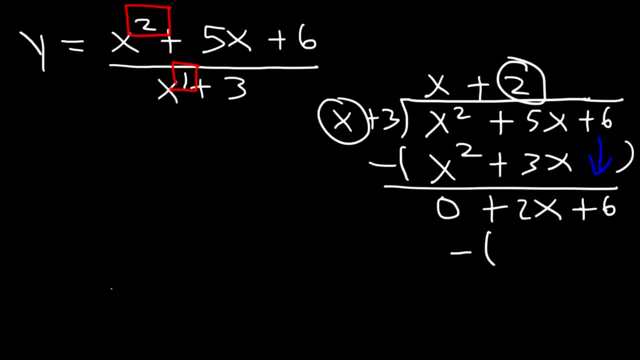 And then let's subtract And then let's multiply. first 2 times x is 2x, And then 2 times 3 is 6.. So there is no remainder. in this case, We're just going to get 0.. 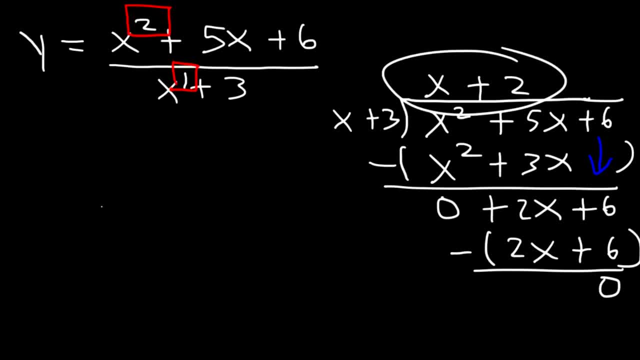 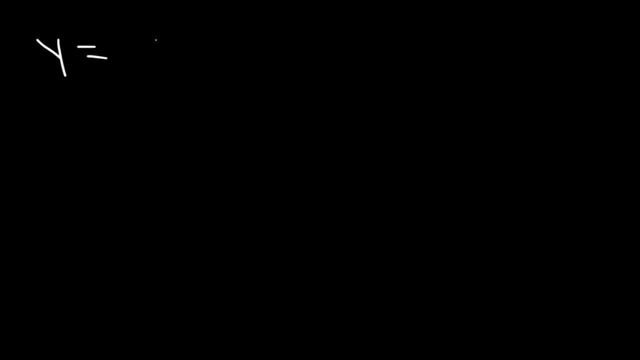 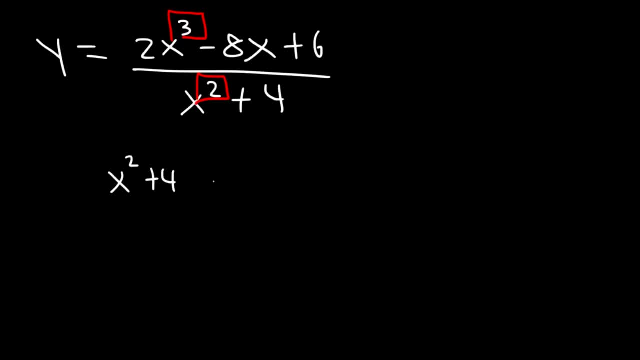 So let's divide. Don't forget about the 0x squared. You need to write that in order to divide it correctly. So let's divide 2x cubed by x squared, That's going to be 2x, And then multiply. 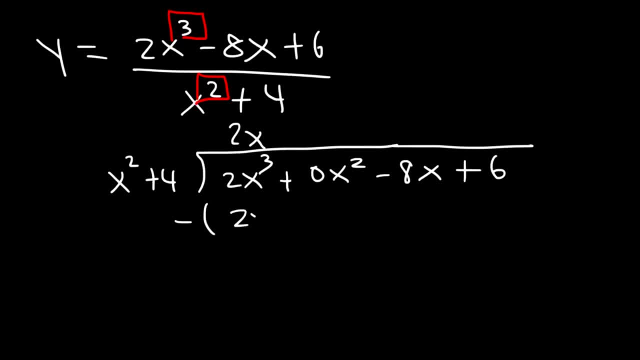 2x times x squared, That's 2x cubed, And then 2x times 4.. That's 8x, which I'm going to put it here. Okay, Okay, Okay, Okay, Okay. Now let's subtract. 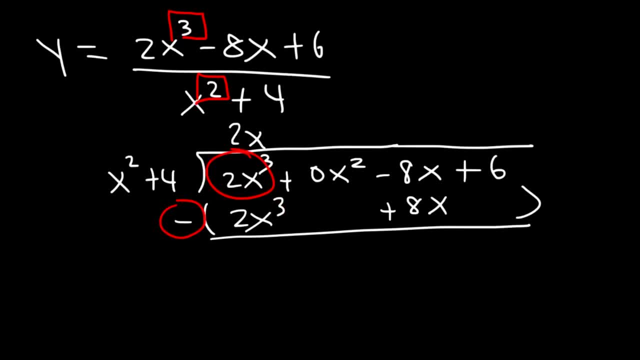 So 2x cubed minus 2x cubed, That will equal 0.. Negative 8x minus positive 8x, That's negative 16x. We can bring down the 6.. So we can't divide negative 16x by x squared. 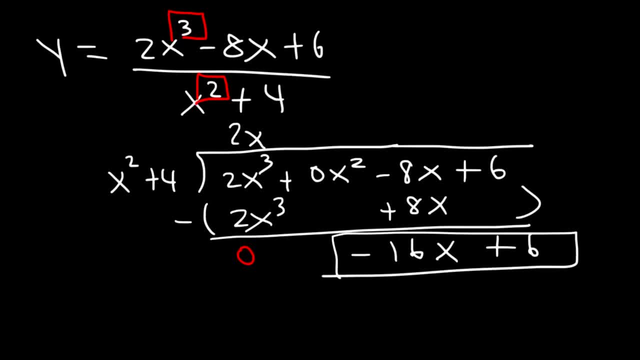 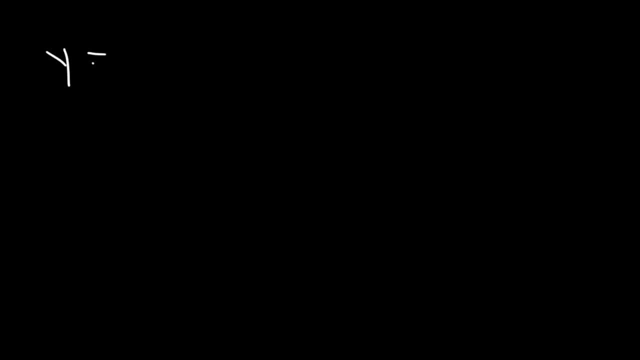 So, therefore, this is the remainder. We don't need to worry about the remainder. The slant asymptote is what you see on here. So the slant asymptote is simply just 2x. Now what about this one? 5x to the 4th minus 6x plus 2 divided by 7x minus 3.. 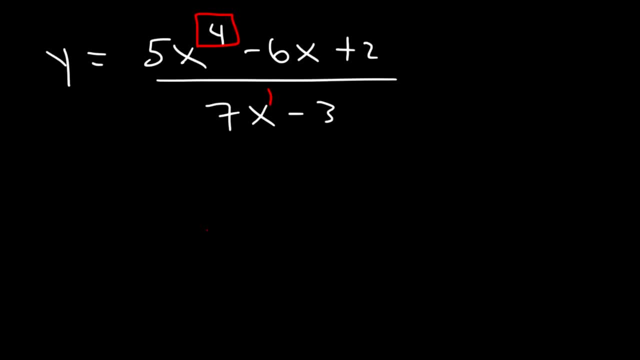 So the degree of the numerator exceeds the denominator by more than 1.. So there is no horizontal asymptote And there's no slant or oblique asymptote. The only time you can get a slant asymptote is if the numerator exceeds the denominator. 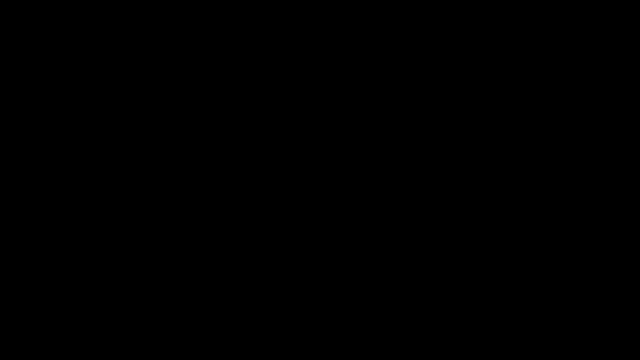 exactly by 1.. So let me give you some practice problems based on the examples that you saw. Go ahead and pause the video and try these. Determine the horizontal asymptote and any slant asymptote. So you will see that the denominator of 1 plus 1 equals the strength of the denominator. 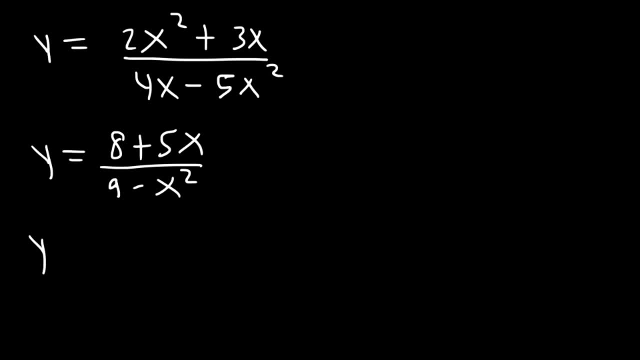 At the end of the line we have the horizontal asymptote. What I'm going to do is just copy this. You can write it down. You will have a connection to the denominator when you get that. We're going to work through this one. On a piece of paper The denominator. So a piece of paper. We're going to put both of them here And we're going to coordinate the denominator And we're going to put them both together And so we're going to write down those numbers. 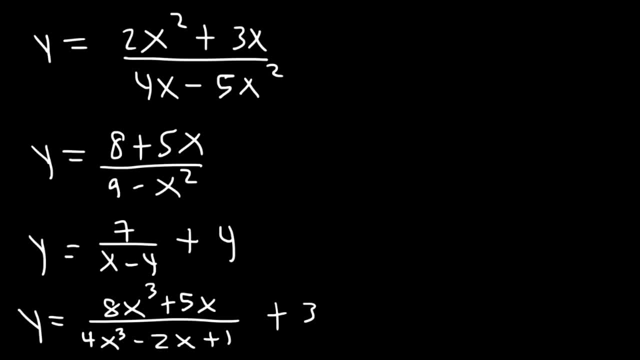 So let's start with the first one. The highest degree is x squared. On top, we have a coefficient of 2 and on the bottom, negative 5.. Both of these are x squared terms, And so it's just going to be 2 over negative 5.. So that's the horizontal asymptote. 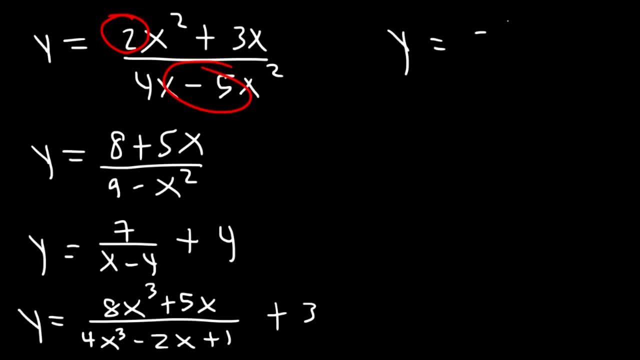 Technically, I should write, y is equal to negative 2 over 5.. Now for the next one. notice that we have a bottom heavy function. The degree of the denominator is greater than that of the numerator. 2 is greater than 1.. So therefore, anytime it's bottom heavy, the horizontal asymptote is 0.. 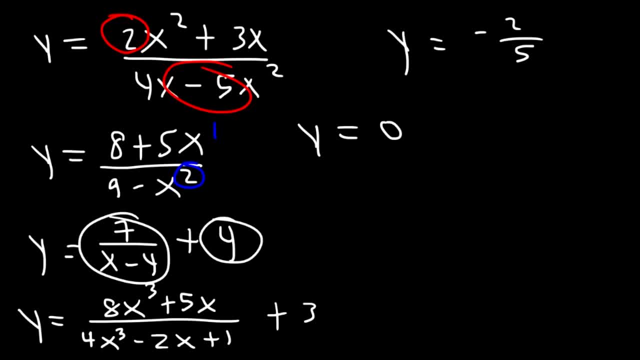 Now this one is also bottom heavy, so that's 0, but we have a plus 4.. So it's going to be: y is equal to 4.. Now in this example, the degree of the numerator is the same as that of the denominator.